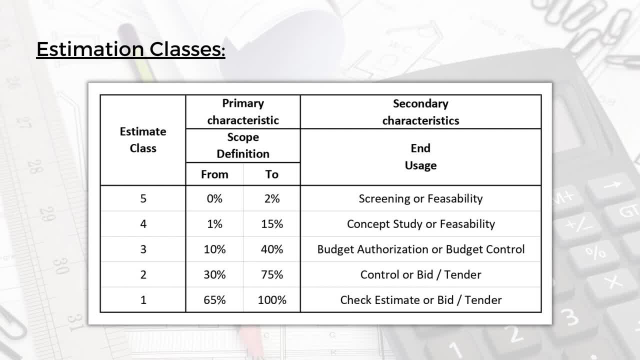 to 100 percent And the ND usage will be check, estimate or bid or tender. So the scope definition will be between 5 to 20 percent to 90 percent, For example. the scope definition will be between 60 percent to 50 percent, For example. the scope definition will be between 60 percent to 80 percent. 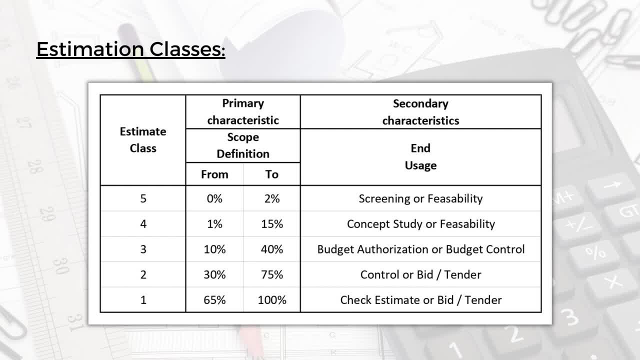 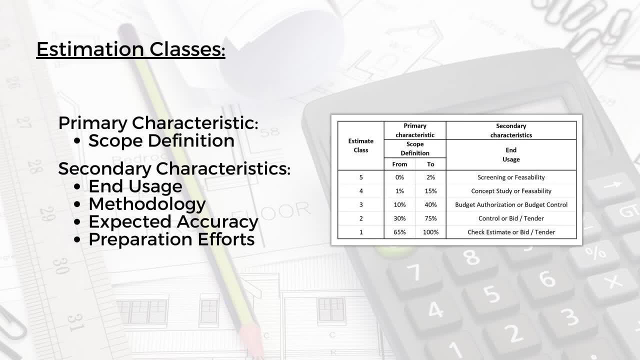 So this is the project. So what we can do with this is we can take the drawings, the specifications and all the project information that we need to produce a very accurate estimate, for example. So if this information are not available or not defined enough, 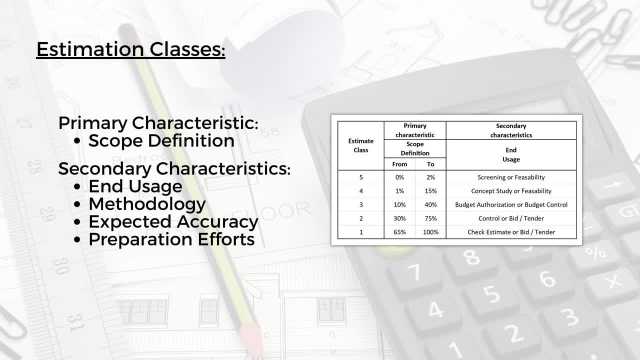 then you cannot produce a class one or class two estimate, but you can maybe produce class three, four or five, something like that. So the take from here is that the primary characteristic is the scope definition. which class of estimate shall we use? the secondary characteristics will be the end usage. why do we? 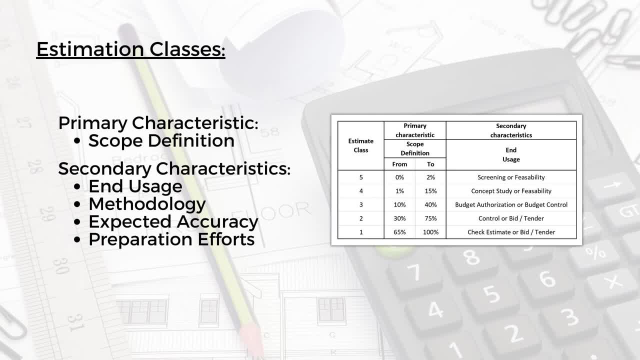 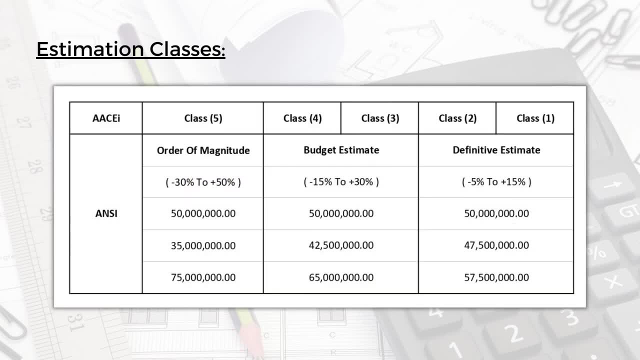 need this estimate. what are we going to do with this estimate and the methodology, which we will be seeing in a moment, and the expected accuracy and the efforts for the preparation as well? so, as we can see here, the estimation classes as per the AACEI, which stands for the association of 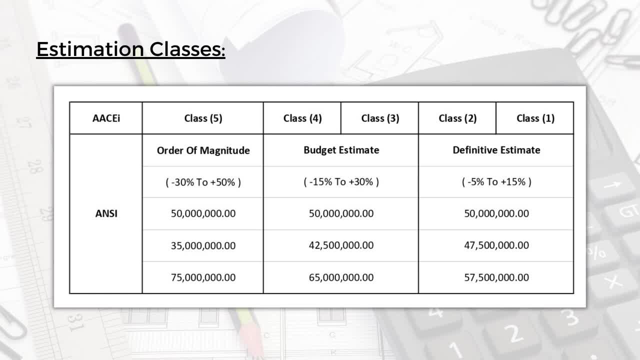 advancement of cost engineering international. they have five classes of estimate: class 5, 4, 3, 2, 1. but as per the ANSI, which is the american national standards institute, class 5 will be equal to something that is called order of magnitude estimate. class 4 and the class 3 will be equal. 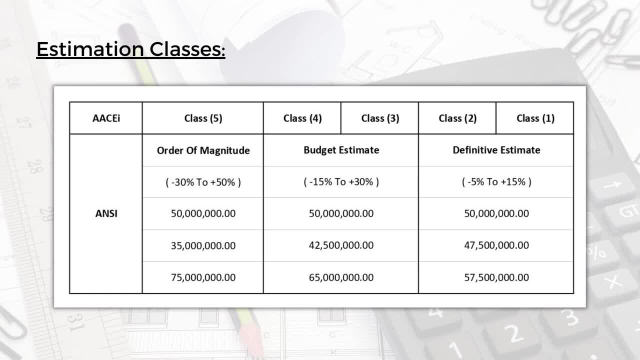 to something called budget estimate. class 2 and the class 1 will be equal to something called definitive estimate and, as per the ANSI, the accuracy of order of magnitude, which is class 5, as per the AACEI, will be between minus 30 percent to plus 50 percent and if we need some numbers, 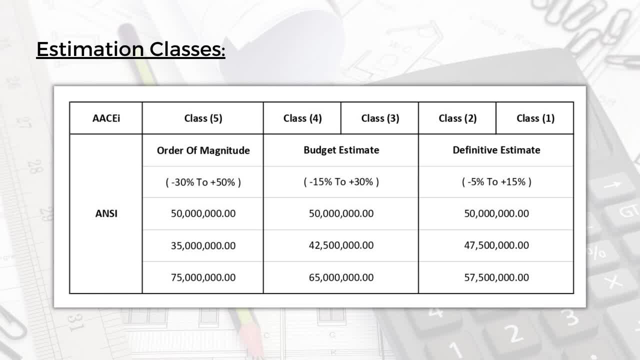 if we need some numbers, we will be able to get the accuracy of order of magnitude, which is class 5. If a building, for example, that is supposed to be a 50 million, when you are doing a class five or an order of magnitude estimate, you can end up with 35 million or 75 million instead of 50 million, because we have an accuracy range of between minus 30 percent to plus 50 percent. 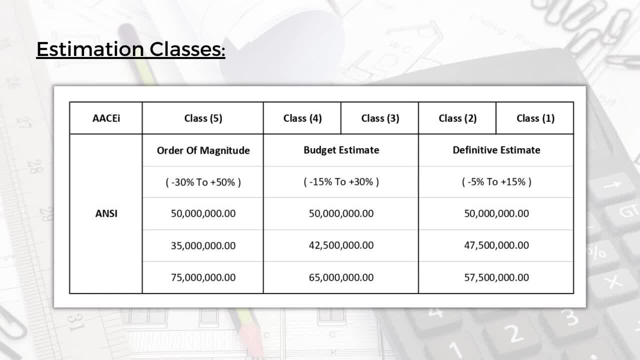 If we are talking about class four and the class three, which is a budget estimate, we will be looking at a range of minus 15 percent to plus 30 percent. So if the building is supposed to be 50 million, you might have an estimate of 42.5 million, or you can have an estimate of 65 million. 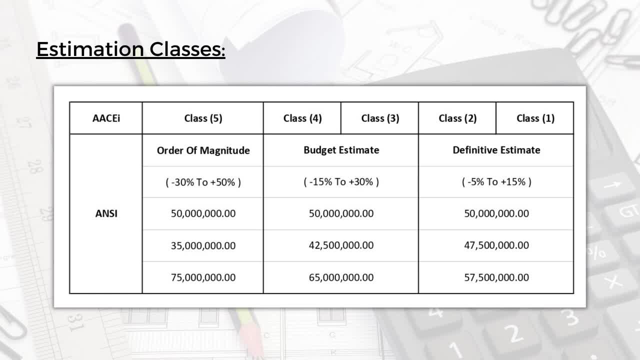 And if we are looking at class two or class one, which is a definitive estimate, we have everything defined and the scope is very clear for us, So we can prepare very accurate estimate, which ranges between minus 5 percent to plus 15 percent. 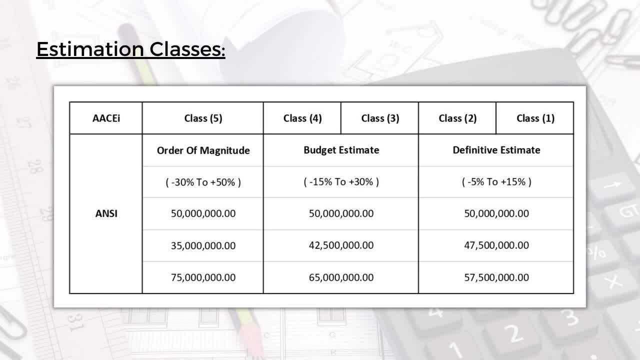 So if the building is supposed to be 50 million, you can have an estimate of 47.5 or 57.5, which are very close to the 50 million. So this is how the AACEI and the ANSI classify, or give us the classification of estimates or the estimation classes. 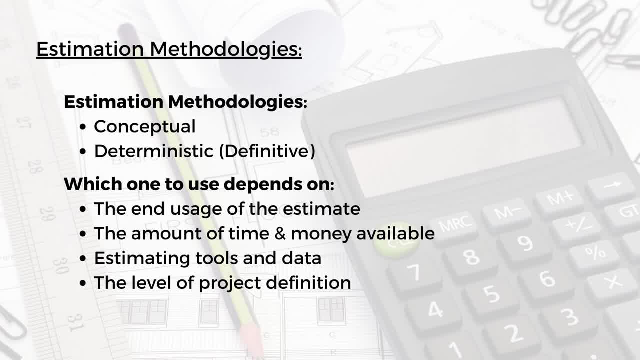 So, when we come to the estimation methodologies, we have two estimation methodologies: We have the conceptual methodology and we have the deterministic or the definitive methodology. And what are these two and what they depend on? This is what we'll be seeing now, But first of all, when to use the conceptual and when to use the deterministic. 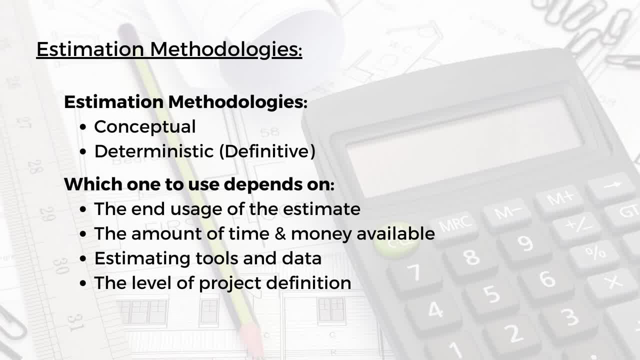 So the usage of any of these will depend On the end usage of the estimate. why do we need this estimate? Is it just a screening or feasibility study, or it's a bid or tender? Why do we need what is the end usage of the estimate and also the amount of time and the money available. 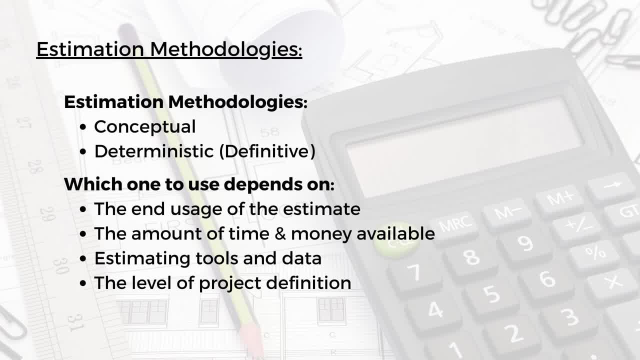 How many resources you have to sit and quantify everything and the estimate everything and get quotations and all of that, Also the tools and the data available and the level of project definition. What are the documents available? Do you have everything- Specifications, drawing, soil report and all what you need to produce a high 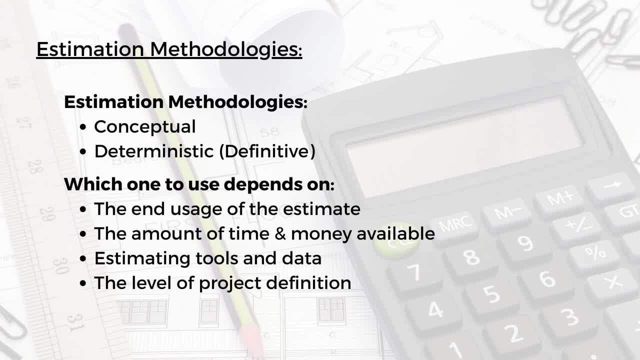 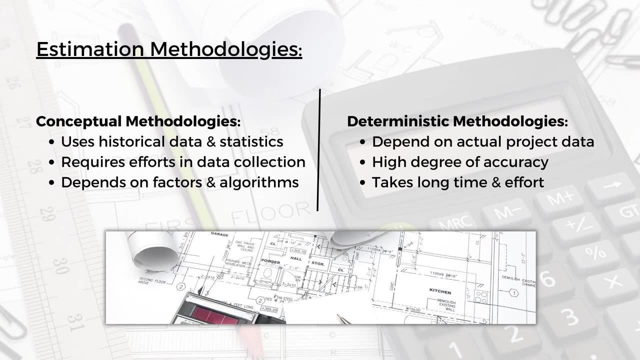 Accuracy estimate or you have just a concept or something like that. So the level of project definition is one of the things that will determine which methodology are you going to use: conceptual or deterministic. So the conceptual methodologies, first of all. these methodologies: uses historical data and statistics, because conceptual means it is not accurate. 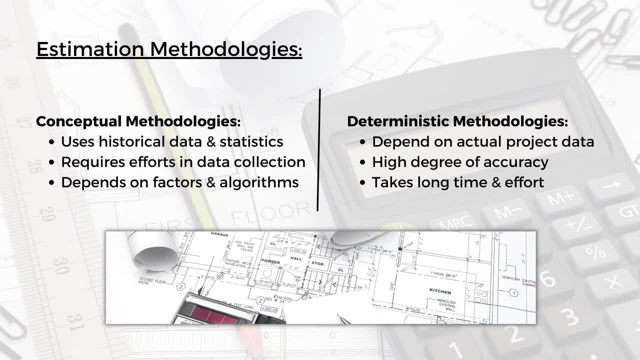 You are just doing some parameters and you are using some historical data and some statistics, and all to produce an approximate value for this project And, as we said, this is very useful When the scope definition is very low or we don't have the scope defined fully yet, so we can use historical data and statistics. 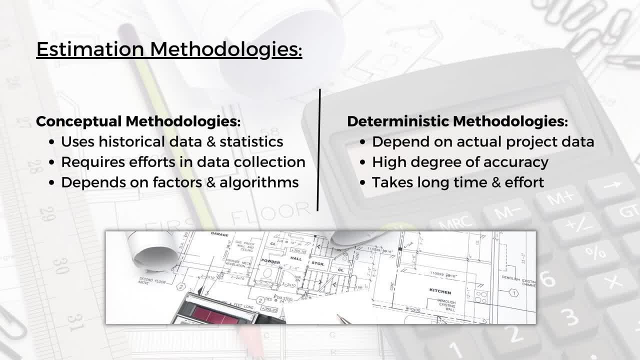 Also, it requires efforts in data collection, but it doesn't require effort in quantity takeoff or gathering the prices from the market and all of this stuff, because we will be using all the projects or historical data to derive the price of this project or the cost of this project. 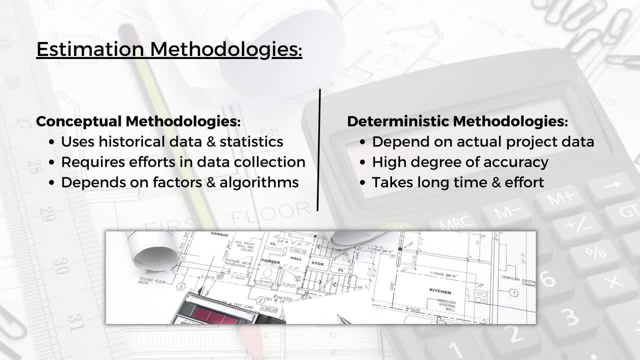 So it requires efforts in the data collection from the past or from your previous project, And also it depends on Factors and algorithms, as we will be seeing now. so it doesn't depend on very accurate estimates and the calculations and accounting and all of that. 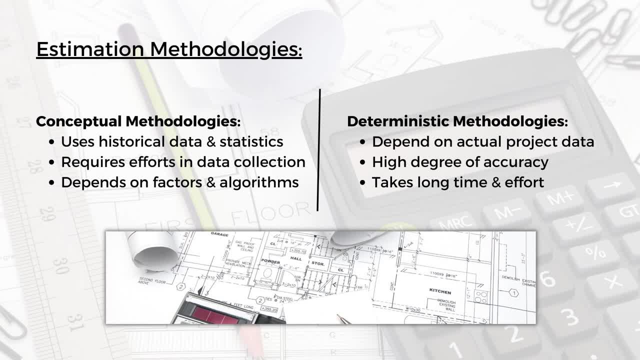 No, it depends on some factors and algorithms. So, when we come to the deterministic methodologies, these methodologies will depend on actual project data, not historical data. No, we have the drawings of the project, the specification of the project itself. So we have the actual project data and that's why we can make a deterministic estimation. 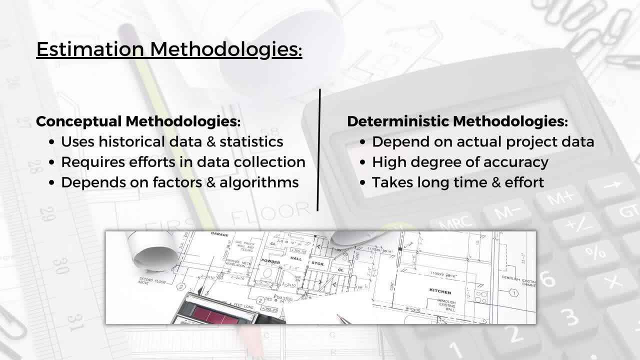 And also it has a very High degree of accuracy because you have all the scope defined in front of you. All you have to do is to price it well or to estimate it very well, and you can get a deterministic estimate. And also it takes a long time and effort to prepare, because you will need to prepare a POQ and you will need to get quotations and incorporate everything and all of that. 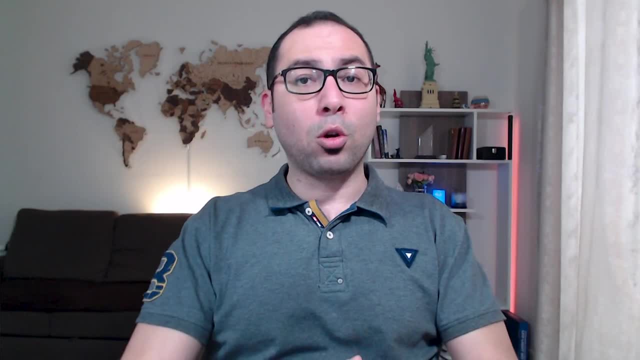 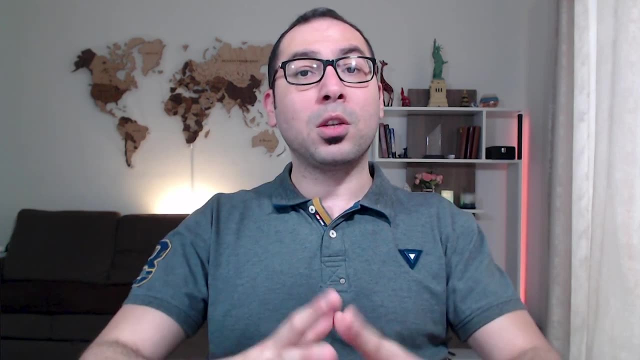 And if we are meeting for the first time- I am Ahmed Adel and you are watching cost engineering professional And here I help you develop the required skills and enhance your knowledge to elevate your cost engineering career. So if this is what you want, 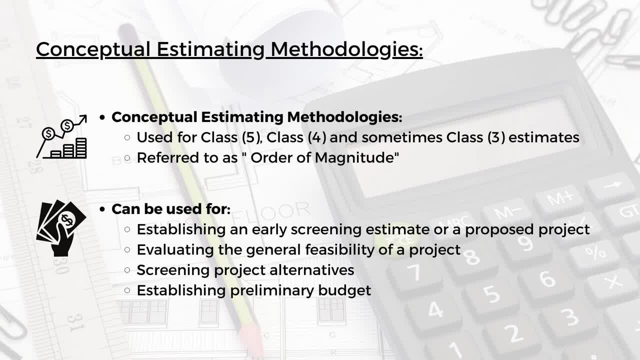 You are in the right place. This channel is for you. So let's talk now about conceptual estimation methodologies. So the conceptual estimation methodologies used for class five and the class four and sometimes class three estimates, And they are also referred to as order of magnitude, as per ANSI, as we have seen previously. 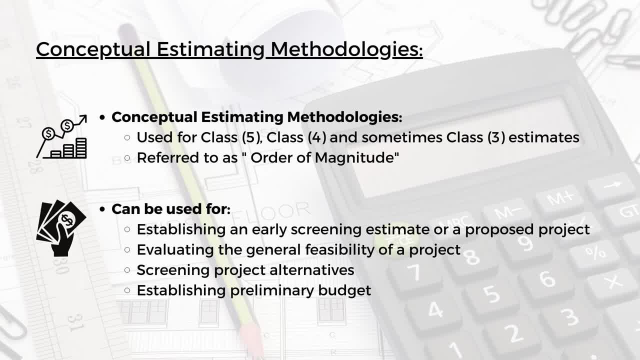 So these are the conceptual estimating methodologies and they can be used for establishing an early screening estimate or a proposed project. So they are being used in the very beginning, when you are just Screening the project or you are establishing a feasibility study or something like that. 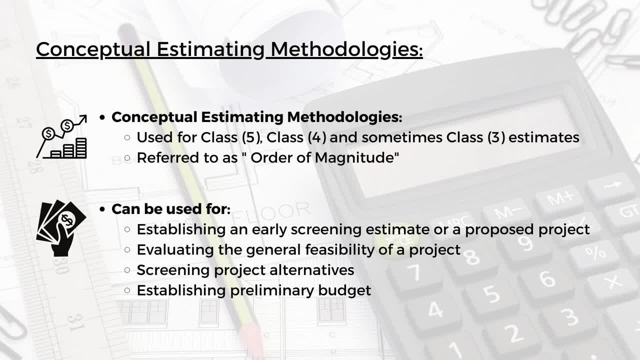 And you can also use them to evaluate the general feasibility of a project, screening project alternatives and also establishing preliminary budget. So, because they are approximate methods or methodologies, they use them only in the very beginning, when the scope is not very well defined, And you can use them for screening, evaluating the general feasibility of a project and project alternatives, budget and all of that. 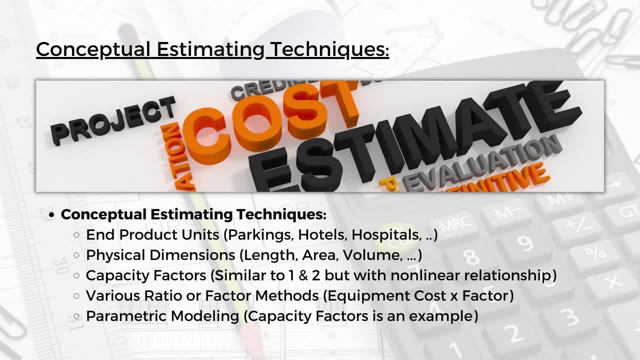 So what are the conceptual estimating techniques Available? We have the first one, the end product units which can be used for projects like multi-story parkings, hotel or hospitals, something like that. So what you will do in this methodology? you will go to an all the project of a hospital, for example, and you will count the number of beds in the hospital. 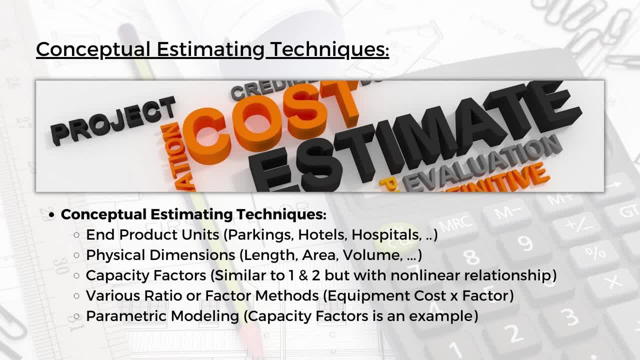 And what was the project value? So you can arrive the bid value, one bid value, and you can apply the same bid value on the project that you have in hand today. You just multiply the bid value by the number of bids that you want to make. 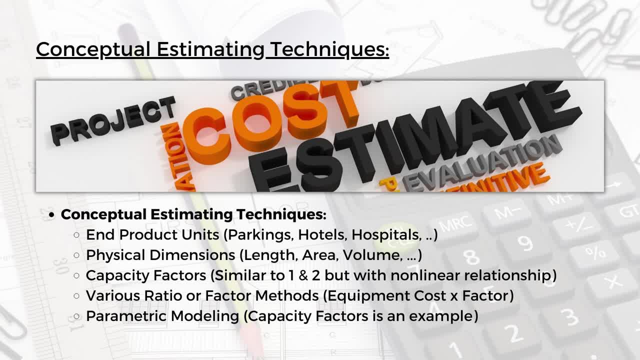 Try it now and you will get the price of this project. So this is the end product unit. Similarly for hotels, how much is the cost per room in our previous hotel project? So today, if we have 1000 rooms, we will just multiply 1000 by the price of room. 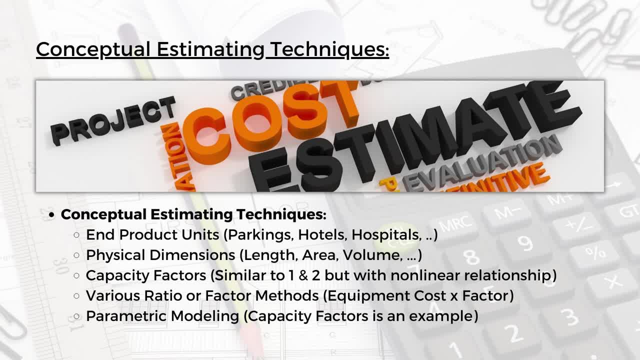 You get the price of the new project Also physical dimensions like length, area, volume and physical dimensions. It can be used for roads or residential buildings, For example. I did in the past a road of 50 kilometers and it costed this much. 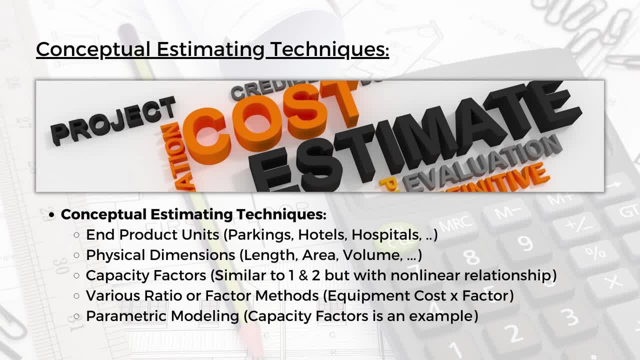 So the cost of one kilometer is this much. So today. if I want to do a road of 100 kilometers, you can just multiply the cost per kilometer into 1000 and you get the price something like that. The same thing is used for residential buildings or villas. 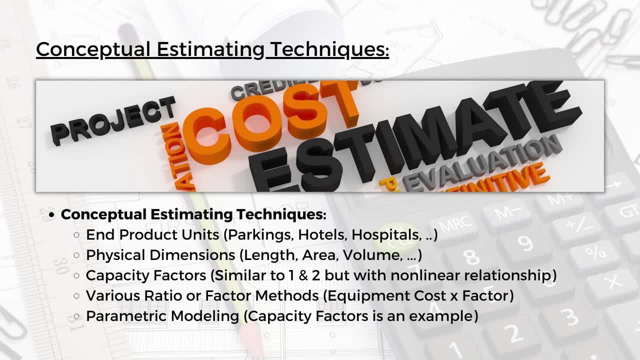 What was the built up area in the past and how much was the cost. So if I am making another built up area, I'll just get the square foot rate or the square meter rate and so on and multiply it by the new built up area that we have to establish the contract price or the approximate conceptual estimating price. 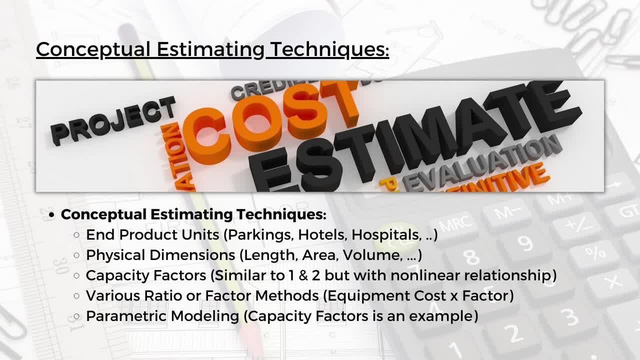 And we have also capacity factors. This is similar to in the product unit and physical dimension, but with nonlinear relationship, And we have also various ratio or factor methods, which is like an example for that can be the FC use or the AC equipments, where you can just say that the cost of fixing an AC unit, along with all the ducts and the grills and everything required, will be the equipment cost multiplied by some factor that you can establish from a previous project. 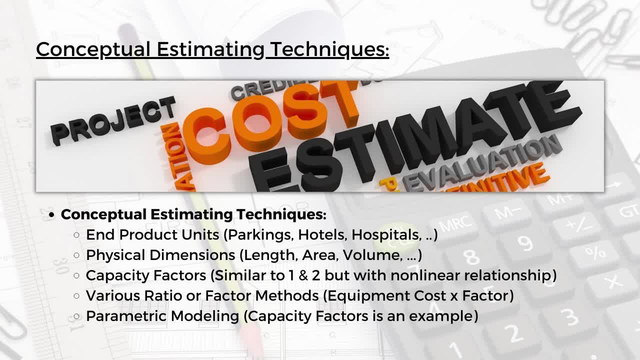 And we have the parametric modeling and actually capacity factor is an example for that Parametric modeling. So these are all conceptual estimating methodologies, as you can see, because they are not giving you an accurate cost estimate for the project that you have in hand, but they are giving you an approximate value only, which can be used for, as we said, preliminary budgeting or feasibility study or project alternatives and stuff like that.